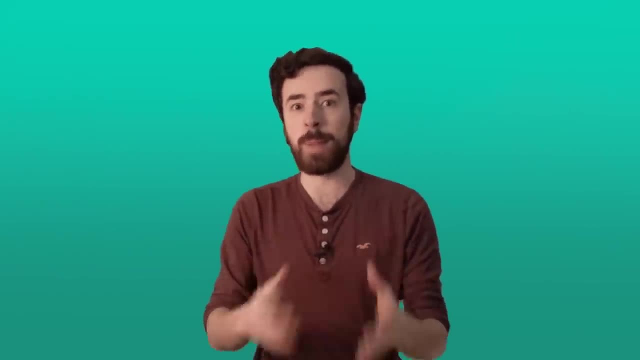 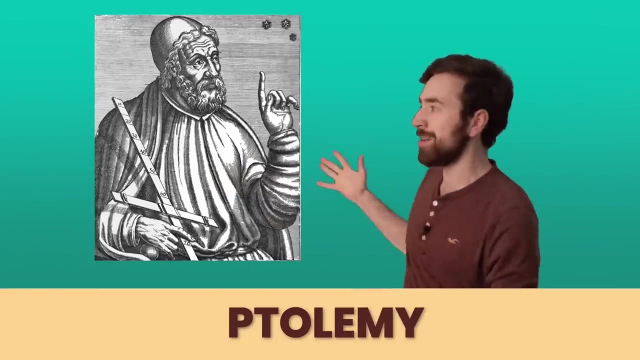 let me tell you about a guy who was really famous in the world of maps. he lived a long time ago and his name was ptolemy. yeah, that's a weird spelling, i know. uh, his name starts with a p, but it's silent, so it sounds like it starts with a t for ptolemy. so ptolemy was one of the most. 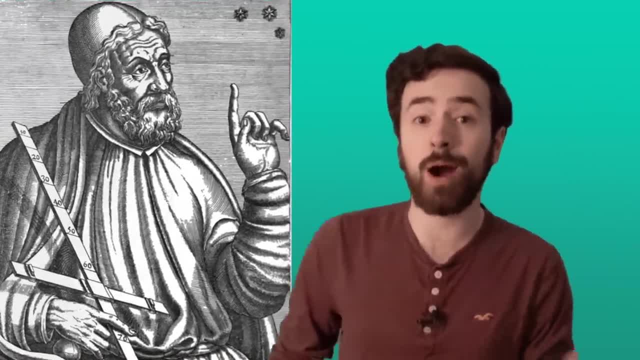 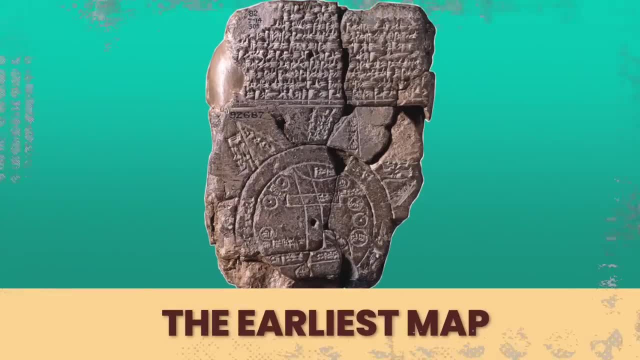 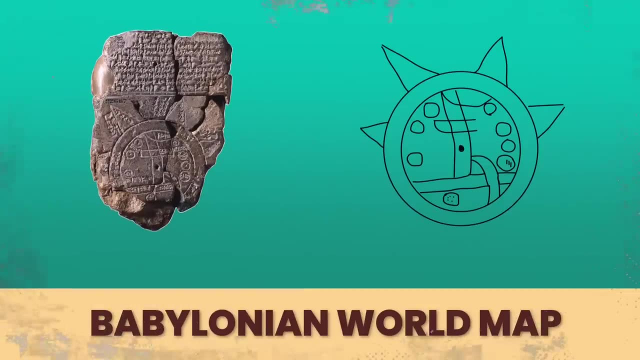 famous geographers who have ever lived, and we're going to talk about how his ideas still help us today. this is one of the earliest and oldest maps we know about. it's clear that maps have changed quite a bit since this one. this is an ancient babylonian map of the world. it was carved on clay and it dates back to about 600. 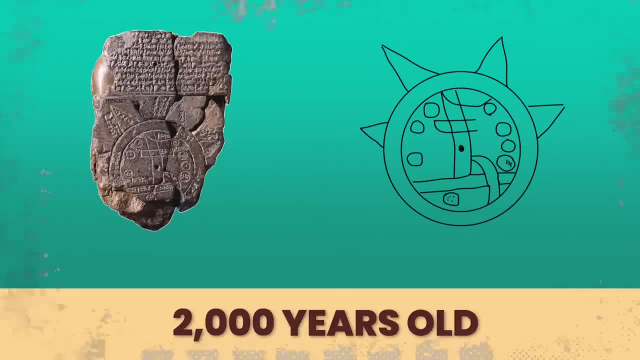 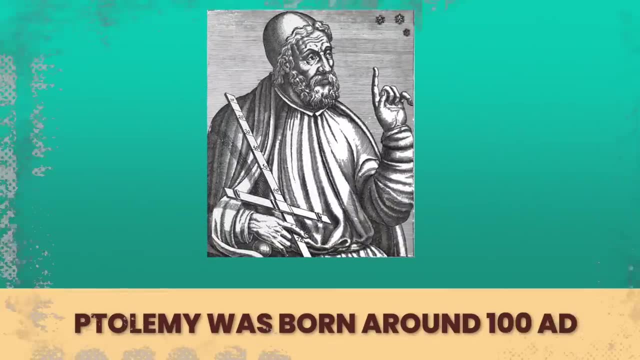 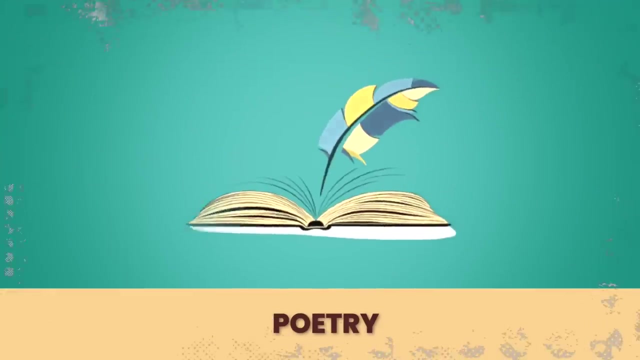 bc. that means it's over 2 000 years old. this is the kind of map that ptolemy worked with. ptolemy was born around 100 ad and he was a roman citizen and he loved math and astronomy and poetry and he especially loved geography. ptolemy gave us something very special. 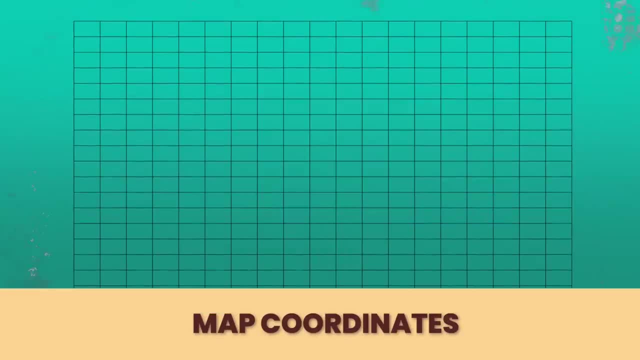 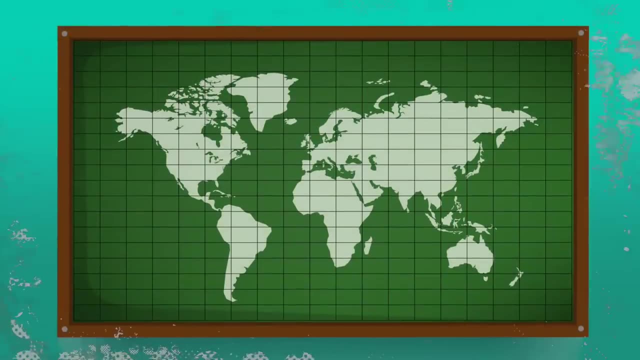 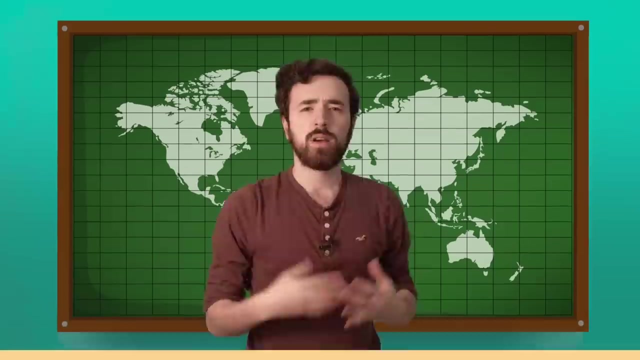 when it comes to maps, he's famous for giving us map coordinates, or those lines we see on the map. we can see them here on a modern day map. the lines that go across show latitude and the lines that go up and down show longitude. have you ever looked in a? 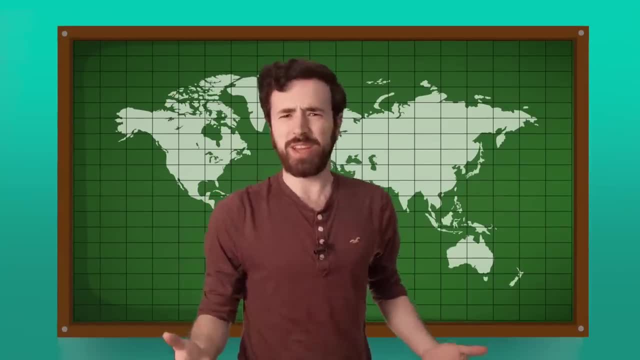 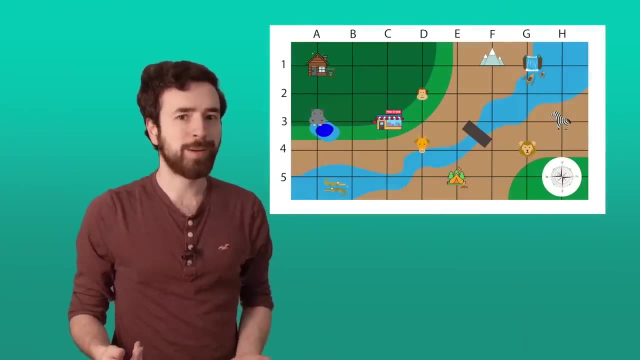 map and thought to yourself: what are all these lines doing here? well, remember the grid or the squares on our safari map. they helped us find our way right. well, these Magθain lines that Ptolemy came up with also help us find our way. The latitude and 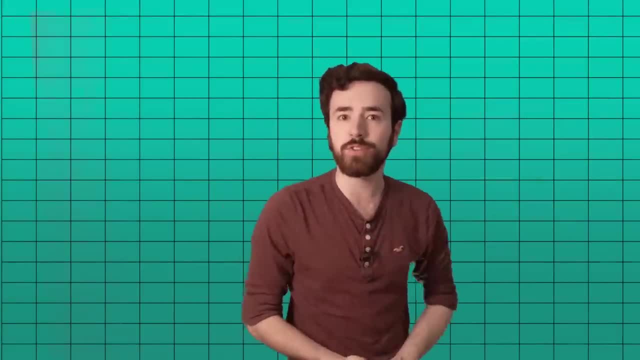 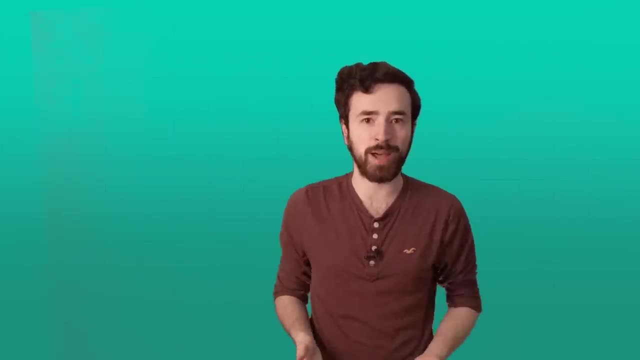 longitude lines for a grid or squares, just like on our safari map. Now, these lines aren't real. You can't go outside and look at the ground and see a line that helps you find your way. But these imaginary lines will still help you when 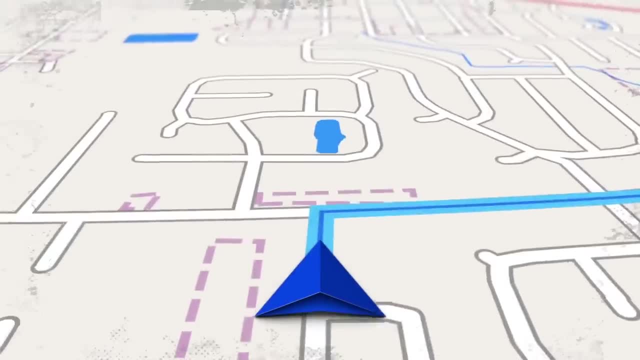 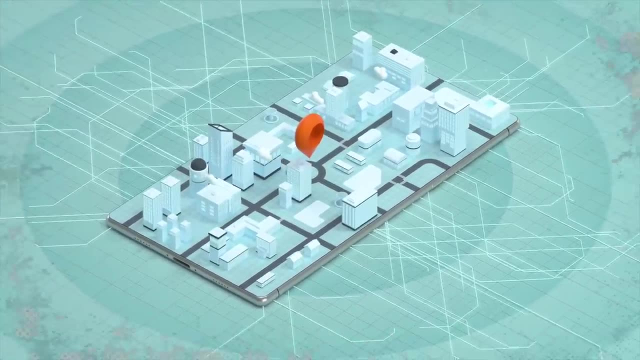 you're reading a map. Today, you can use a GPS system in your car or on your phone to figure out where you are, But it hasn't always been that way. We've always been able to figure out where we're going or where we are thanks to these. 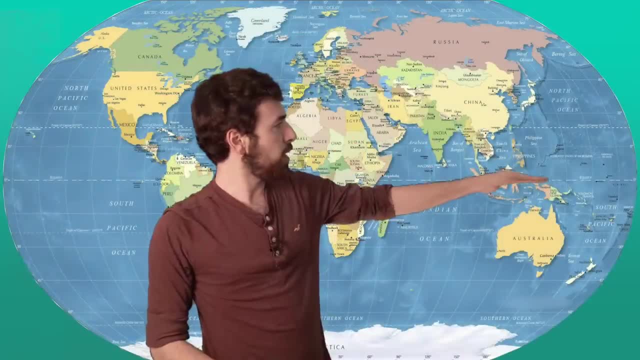 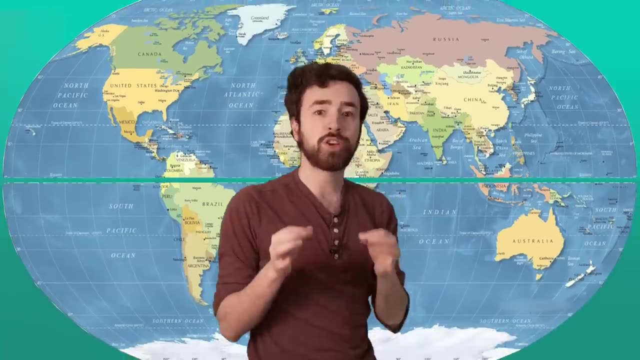 lines that Ptolemy came up with. This big imaginary line runs right through the middle of our map. It's almost like it's cutting the earth in half. This line is called the equator. This area above the equator is north of the equator and the 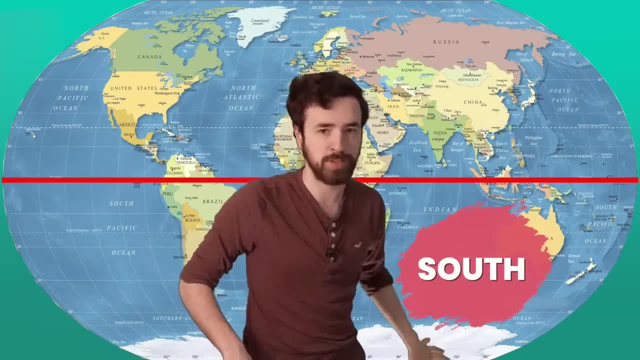 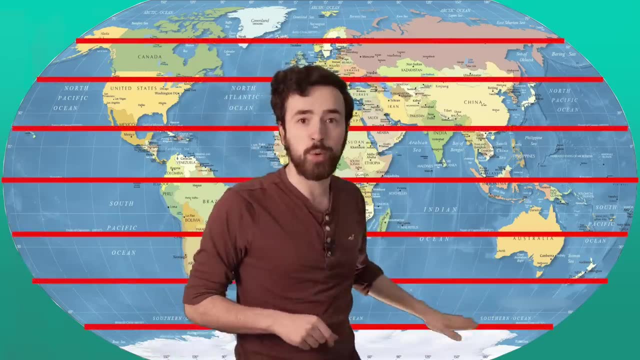 area down below the equator is south of the equator. Okay, here's where it gets good. These lines that run north of the equator and that run south of the equator are called the equator, And these lines that run south of the equator are called latitude lines. Hold your arms out like. 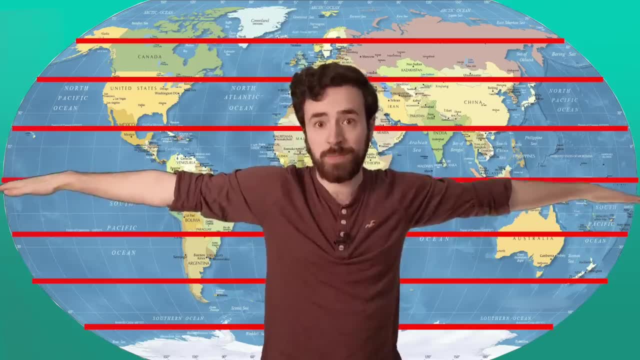 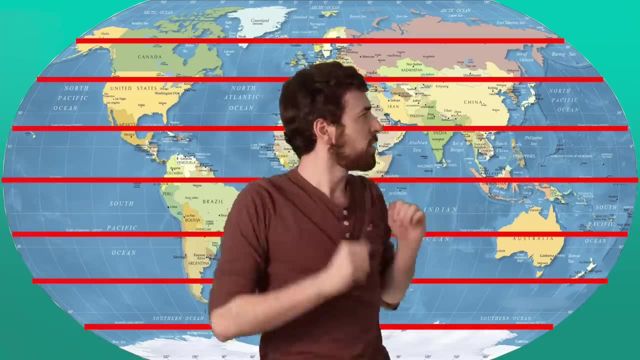 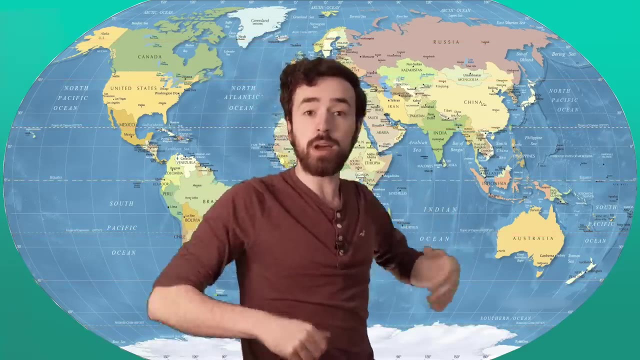 this. This is the way that latitude lines run Across. You can also just say: lat lines are flat lines. Can you see how the lines are numbered? from 0 to 90 in this map? The 0 and 90 are coordinates, just like on our safari map Every. 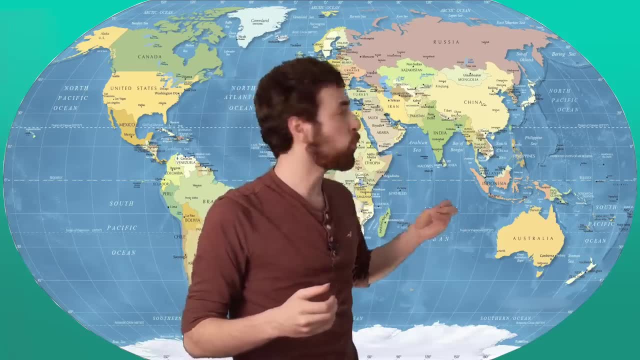 latitude line has a number as well as a number, So you can see how the lines are numbered, from 0 to 90 in this map. The 0 and 90 are coordinates, just like on our safari map. Every latitude line has a number as well as. 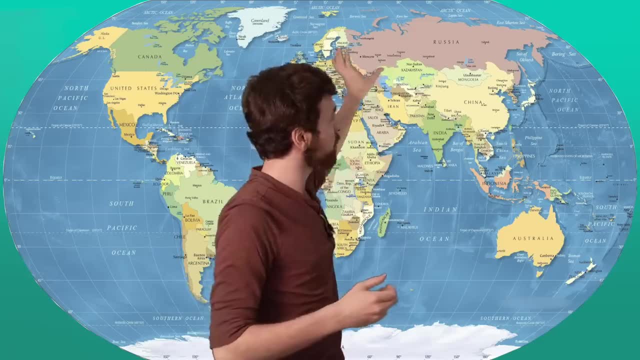 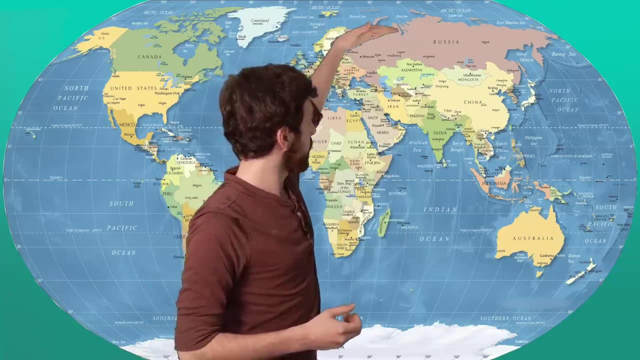 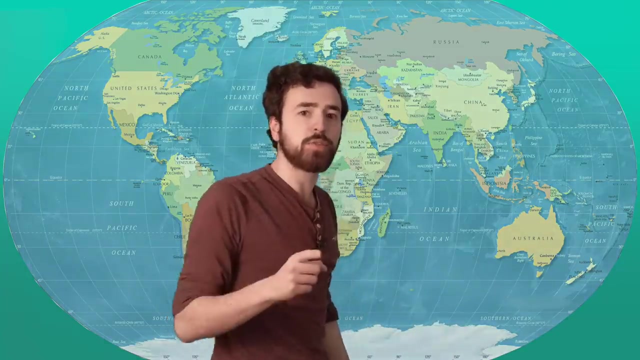 a letter: N to show that it's north of the equator, or S to show that it's south of the equator. Moving up from the equator is moving north, and moving down away from the equator is moving south. Stay tuned for more info on Ptolemy's imaginary. 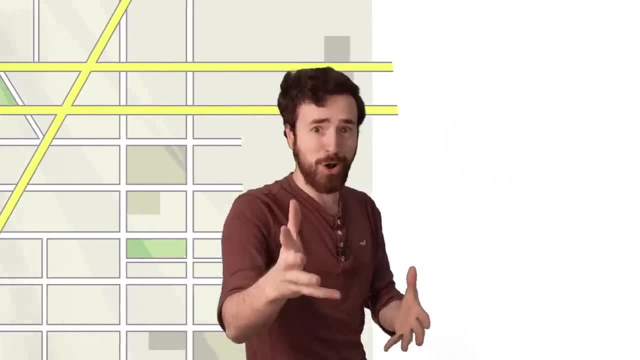 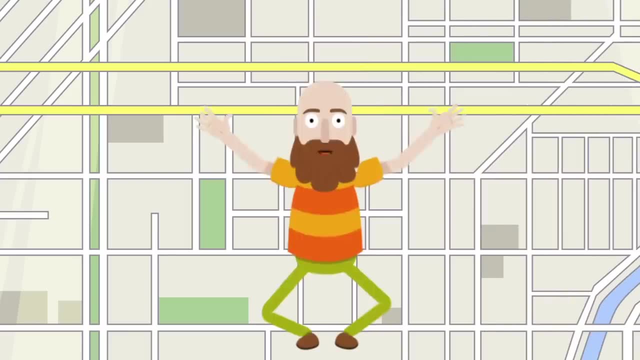 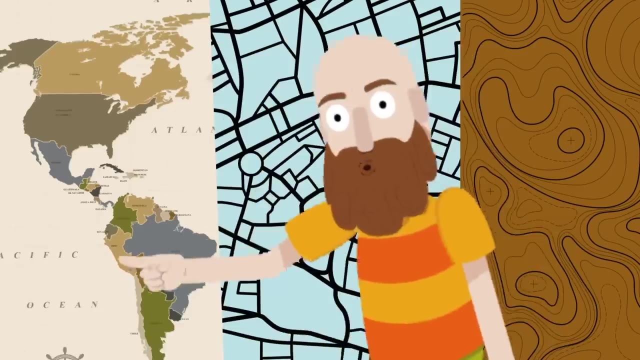 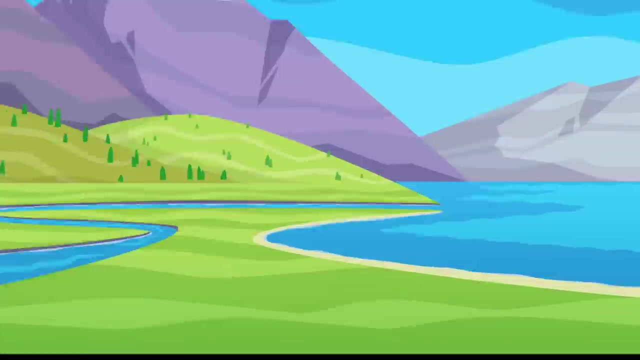 lines. but first it's time for our map rap. A rap about maps. A rap about maps. North, south, east, west. I look at a map when I'm on my quest. Where am I going? What's the map showing? Is there a lake or a mountain Or a river? 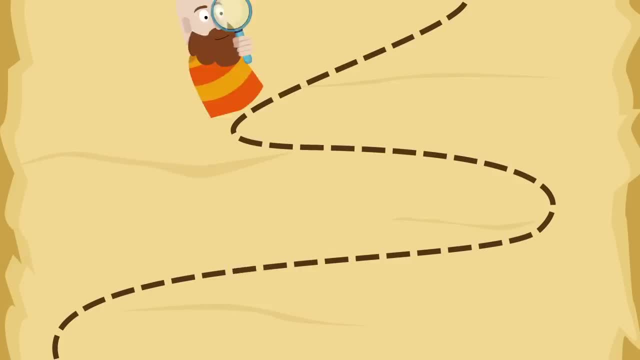 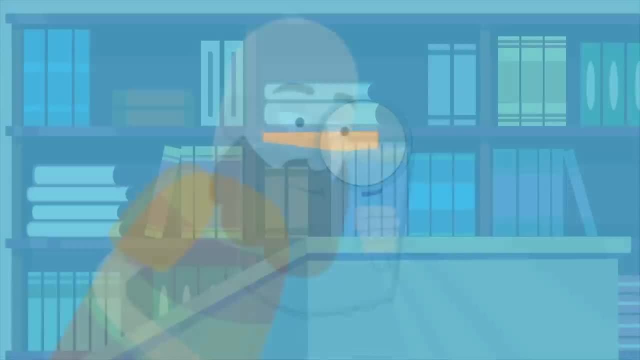 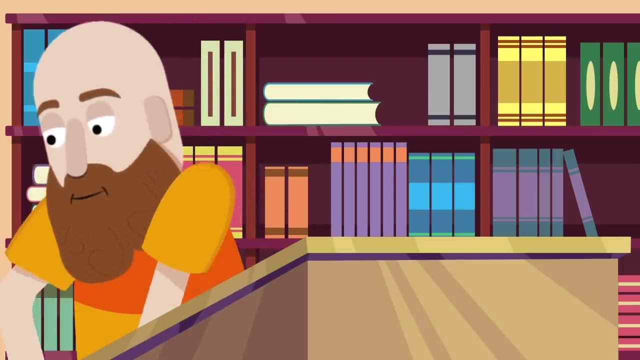 that's flowing. It's a rap about maps. A rap about maps North, south, east, west. Tuck it in my pocket when I'm wearing a vest. Knowing how to read a map. Now, that's the key. I've got a few handy. come on and follow me. 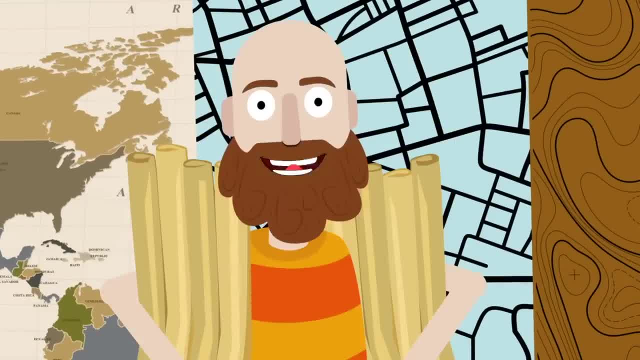 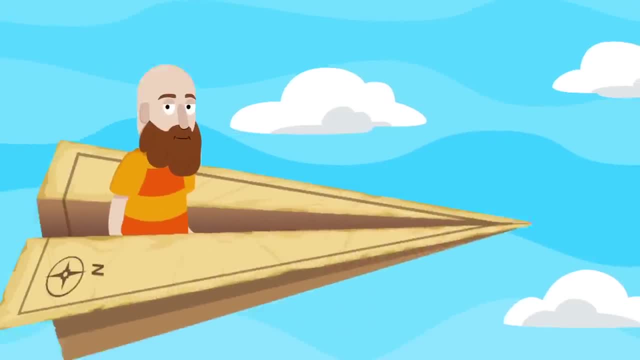 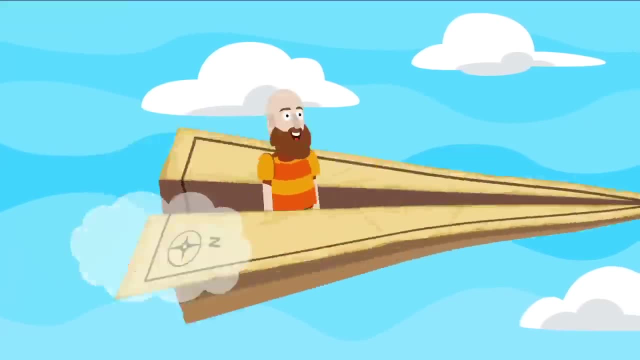 Maps, maps. I love to read them, Maps, maps, I love to hold them. Maps, maps, maps, maps, and everybody has trouble trying to fold them. It's a rap about maps. A rap about maps- North, south, east, west. when you're on your journey, maps are the best. 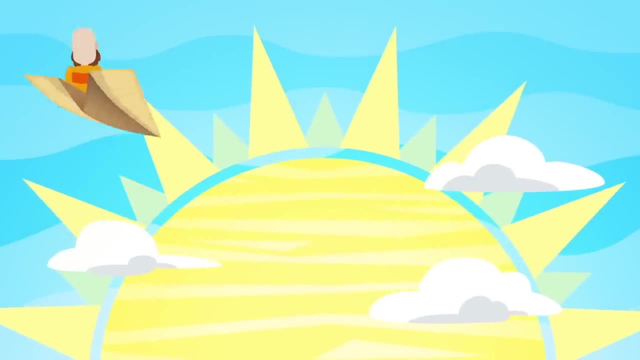 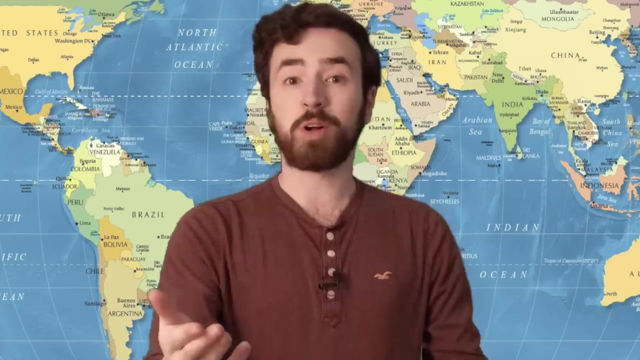 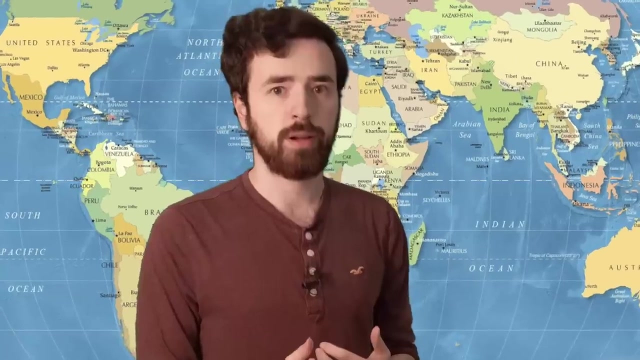 That's a rap about maps. A rap about maps. Welcome back Now. before we were talking about latitude lines that run north and south of the equator. Now we need to add our east and west part of our coordinates. This is the prime. 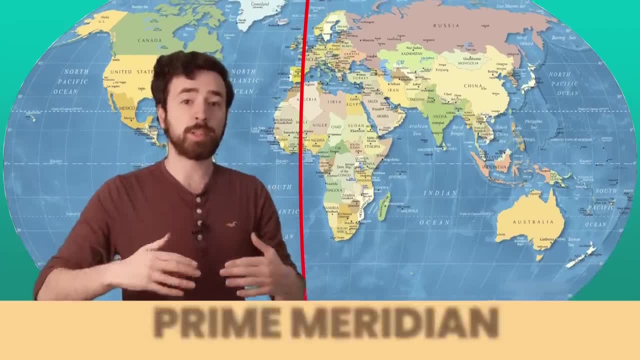 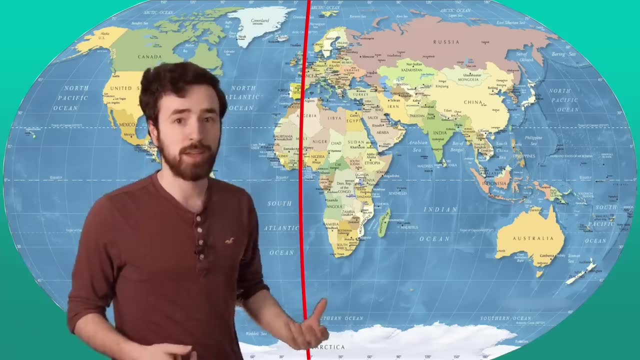 meridian. The equator is a line that divides our map into north and south. The prime meridian is the line that divides our map into north and south. The prime meridian is the line that divides our map into north and south. The prime meridian is a line that divides our map into east and west. It also has a 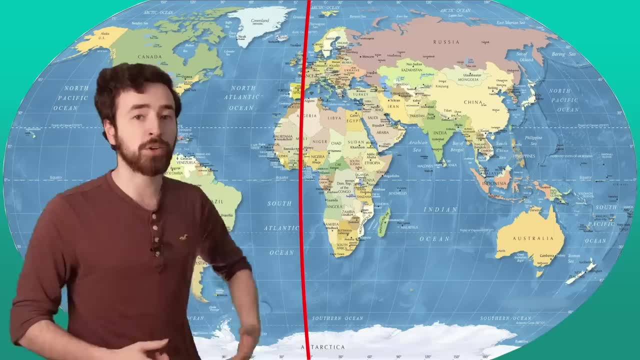 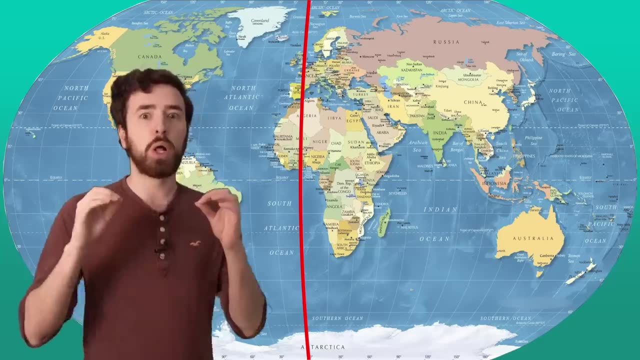 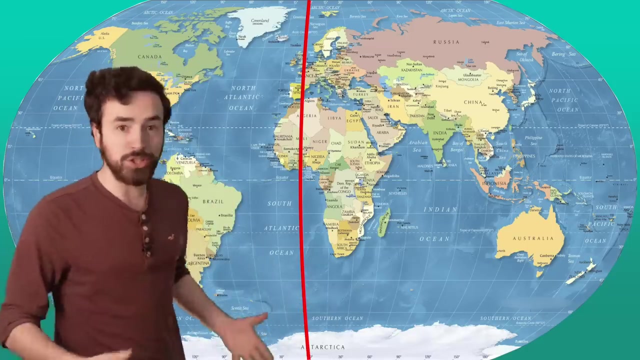 coordinate of zero Longitude lines are the lines that run east and west of the prime meridian. An easy way to remember which way longitude lines go is the word long. Longitude lines are long. The long longitude lines go east and west of the prime meridian and they go from 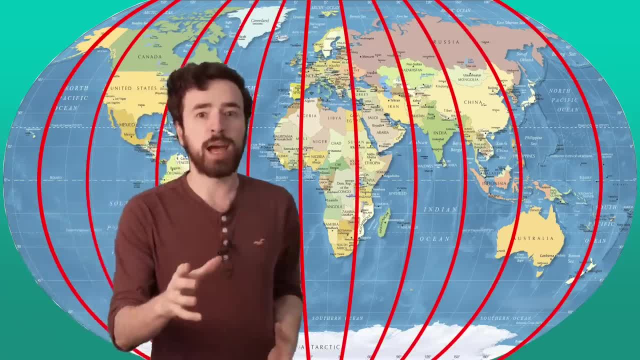 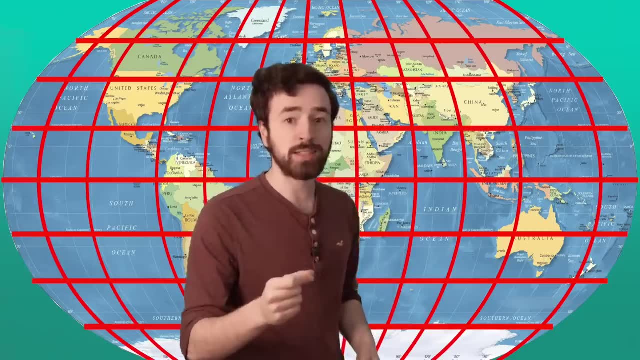 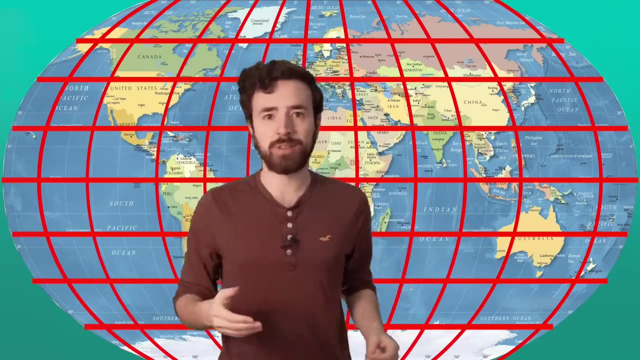 aOC to a D from the long longitude line to A from the upper side of the synonym. but longitude lines don't go that far either. Okay, so if we take ourこれで 180 coordinate? okay, now it's time to put our latitude and 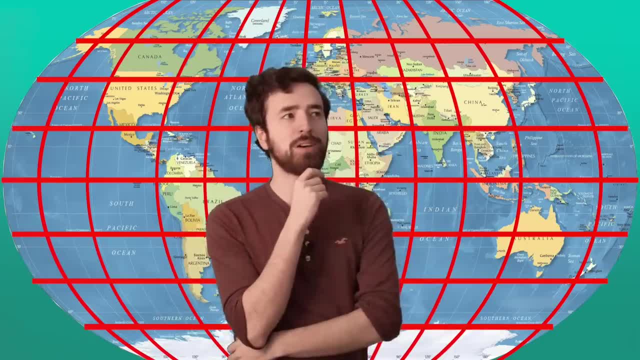 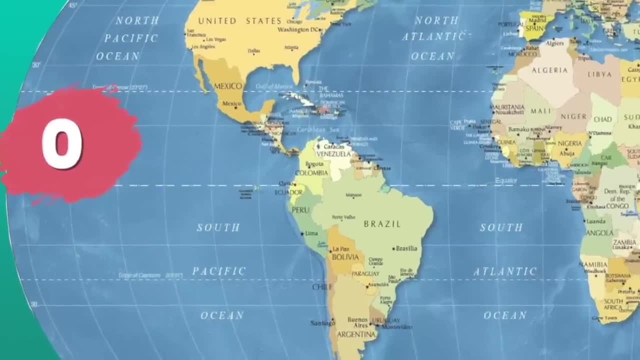 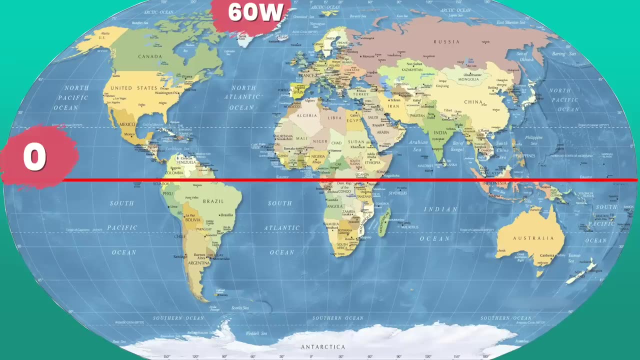 longitude lines together. If we use our latitude and longitude lines and our coordinates, we could find any location on the map. mystery location are zero and 60 West. Remember we look for latitude first, because latitude has an attitude. if we don't, 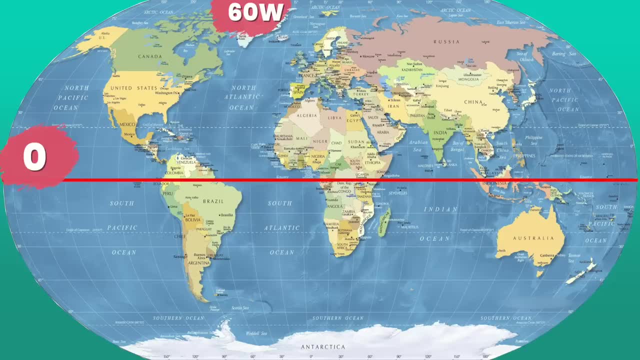 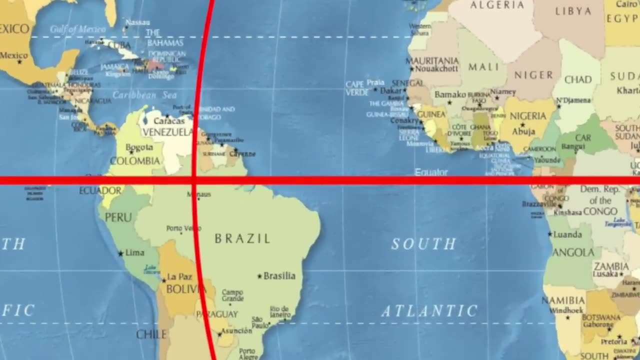 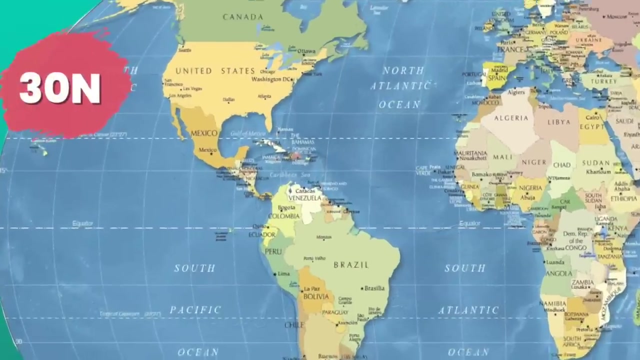 Here is our latitude line at zero. Next, let's find 60 West, which is the longitude line. Follow the lines. Where do they lead us? Brazil, Our next mystery location is 30 North and 30 East. Don't forget latitude first. 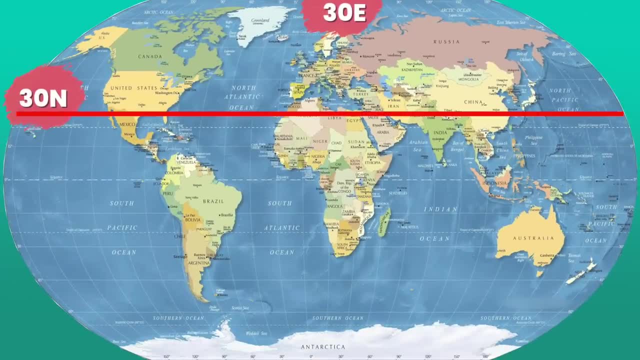 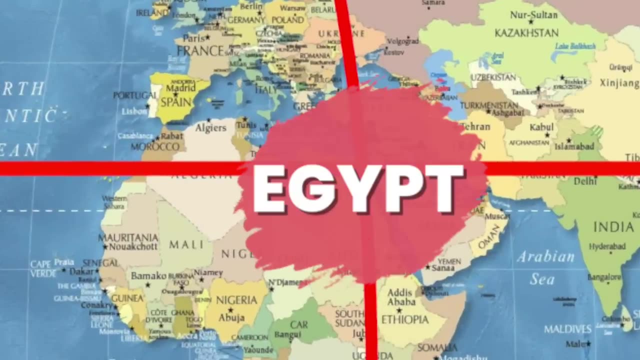 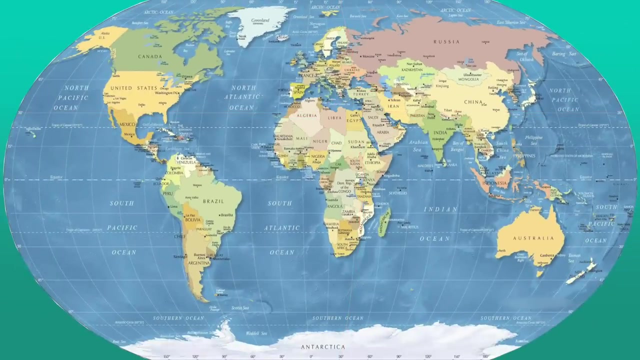 So 30 North is our latitude, Then 30 East is our longitude. Where do they meet? Egypt, All right, one more. Now you're becoming an expert at this. Here we go. Latitude is 30 South and longitude is 135 East.